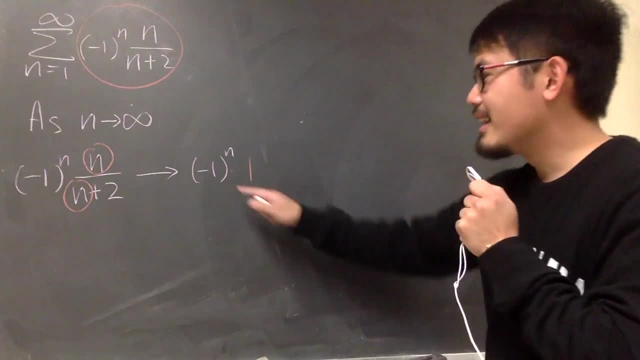 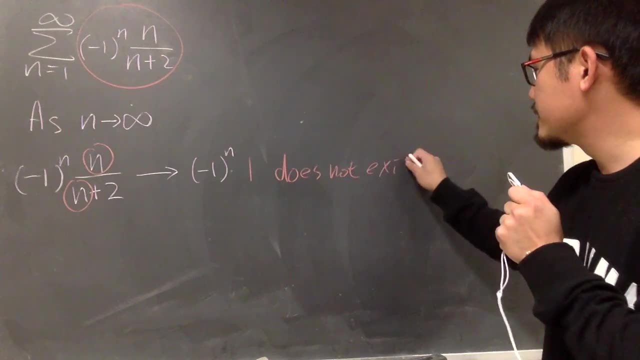 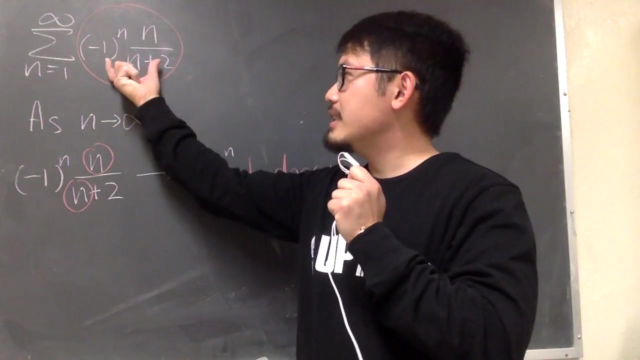 So this will never approach to a number. right This right here. the limit of this does not exist, which is enough. okay, Once again, as long as you take the limit of this AM formula, as long as this is not approaching to 0, we are good. 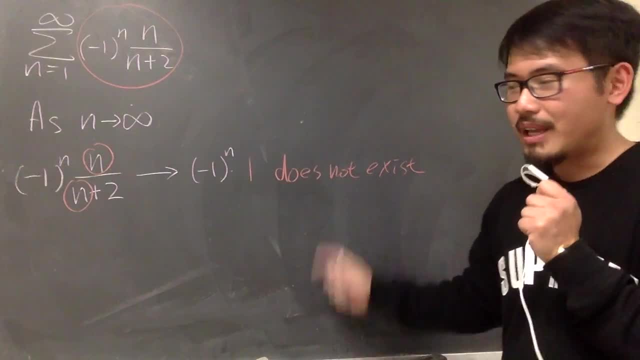 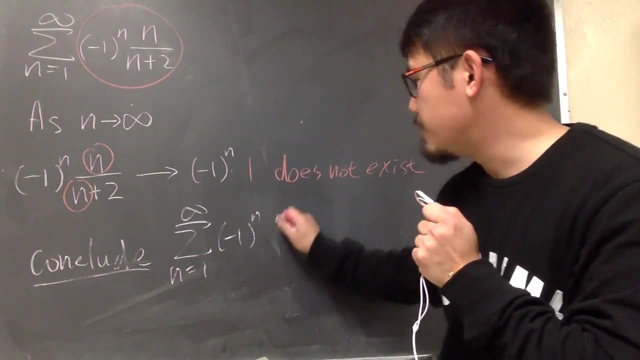 including does not exist situation like this. So I can conclude. let me just write it down. We are going to conclude that the original series, sigma as n, goes from 1 to infinity negative 1 to the nth power, n over n plus 2.. 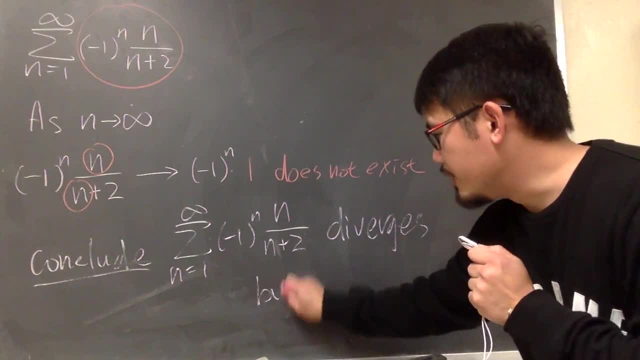 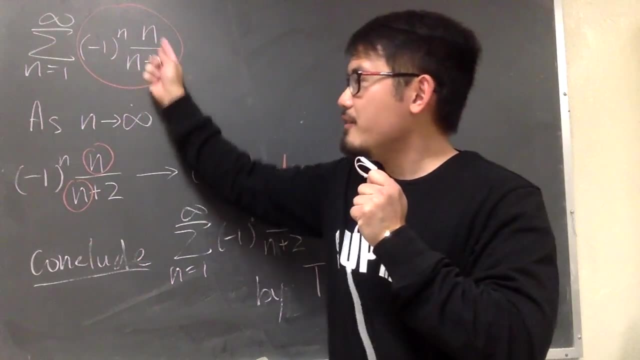 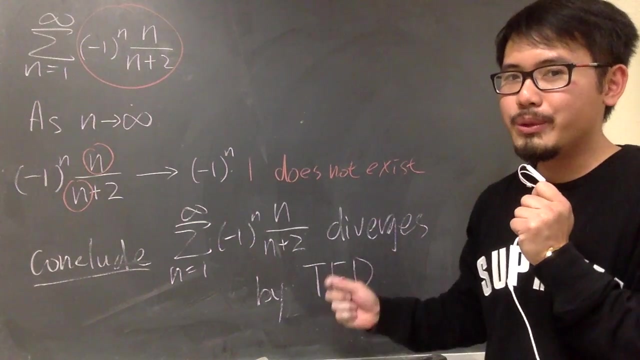 This right here diverges And we know that. it's because by the test for divergence One more time, as long as the AM formula does not approach to 0, then we can argue that the series diverges, including the situation that when you have this limit being non-existent, 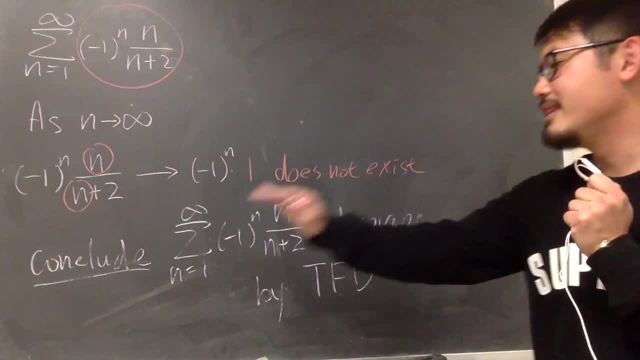 This does not exist. we are good To say the original series diverges by test for divergence, That's it. 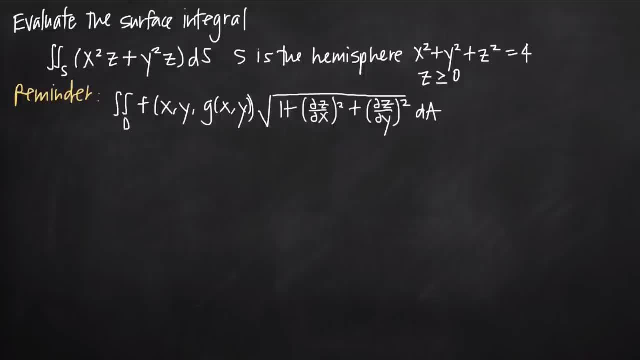 In this video we're going to be talking about how to evaluate a surface integral, And in this particular problem we've been asked to find the surface integral of the function x squared z, plus y squared z- ds, where s is the hemisphere given by the equation x squared. 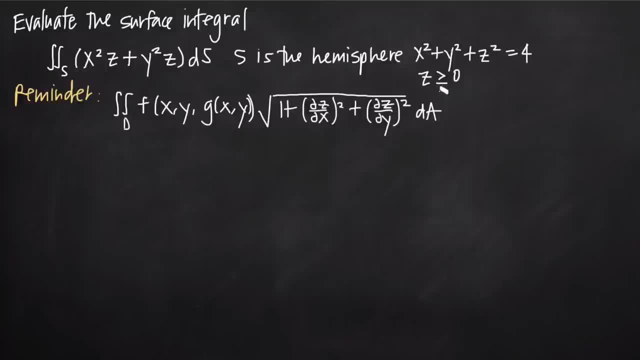 plus y squared plus z squared equals 4 and by the inequality, z greater than or equal to 0.. So the first thing we want to realize is that our equation here that defines s is x squared plus y squared plus z squared, which is the standard equation of a sphere where 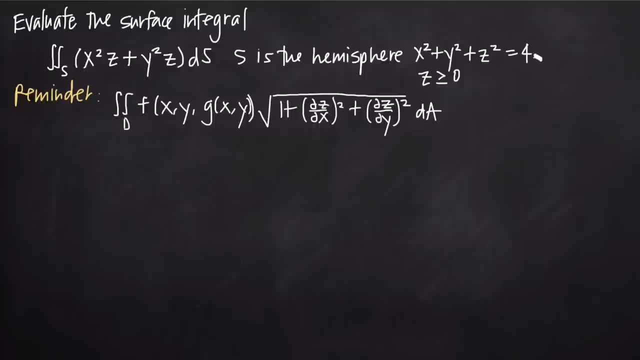 the square of the right hand side over here is the radius. So normally, if we just looked at this equation on its own, we'd have the equation of a sphere in three dimensional space centered at the origin with radius 2.. But we've also been told that z has to be. 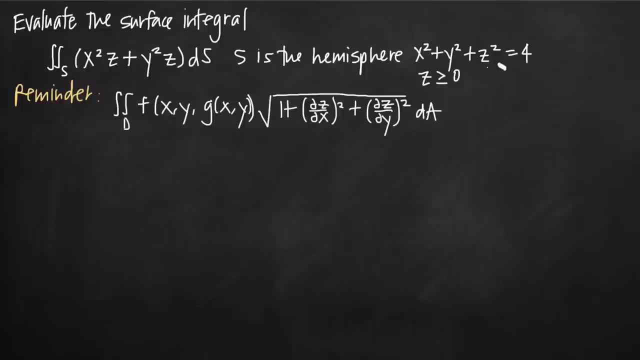